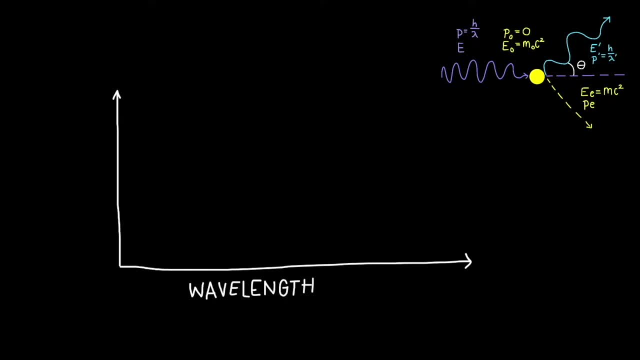 If we plot the photon's wavelength on a graph, we'll notice that its intensity peaks at a certain wavelength. If we plot the photon's wavelength on a graph, we'll notice that its intensity peaks at a certain wavelength, as indicated by the purple curve When it scatters. 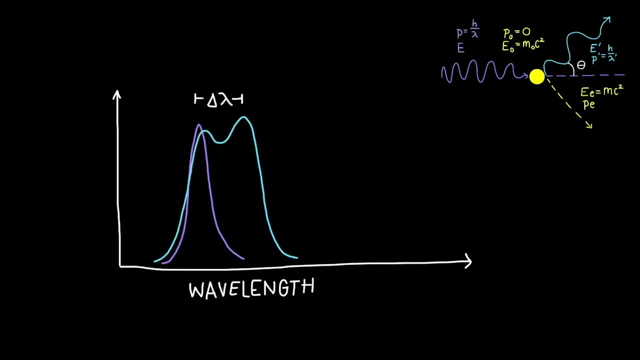 there will be a shift in the wavelength, with another peak at a wavelength higher than the first. The amount that this wavelength shifts is dependent on our scattering angle: theta. When theta increases, the change in wavelength increases. The standard form of the Compton. 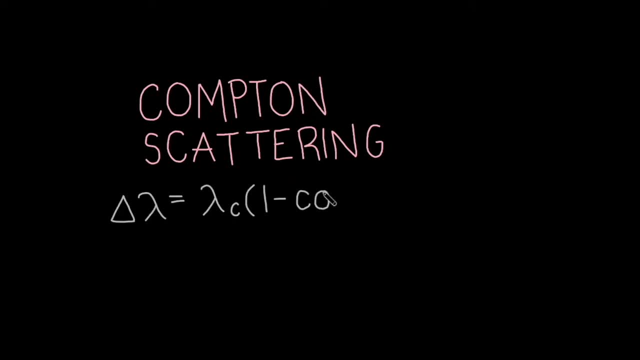 equation is: the change in wavelength is equal to the Compton wavelength times one minus cosine theta. But how do we get there from this scenario? We will use two important conservation rules: The conservation of energy and the conservation of momentum. That and a whole lot of algebra. 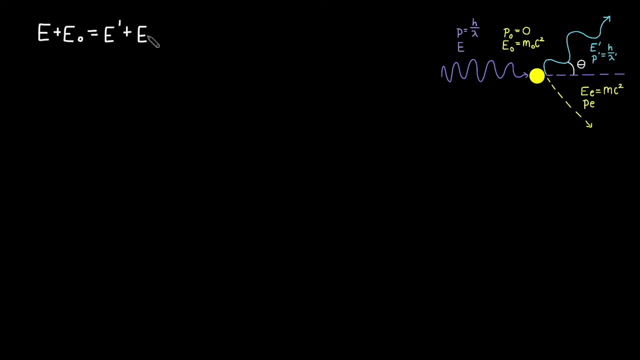 Let's start with the conservation of energy. The energy of a photon and the electron before collision is equivalent to the energy of the photon and electron after collision. We can substitute what we know about the electron's initial energy in for e naught. Now let's arrange everything so that we isolate the photon's final energy on the 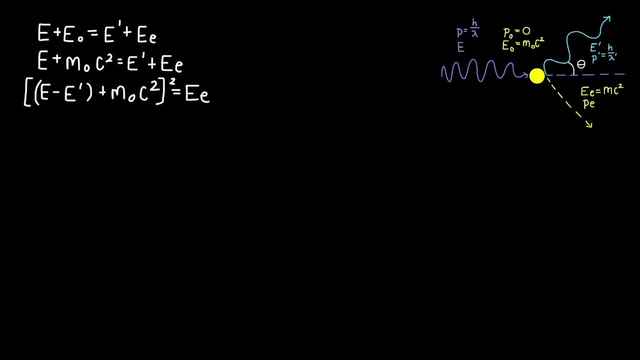 right-hand side of our equation and square everything. Now, some of these algebraic manipulations may seem arbitrary. Remember, we are focused on rearranging our equation in such a way so that we eventually derive the Compton equation If we divide everything by c squared. 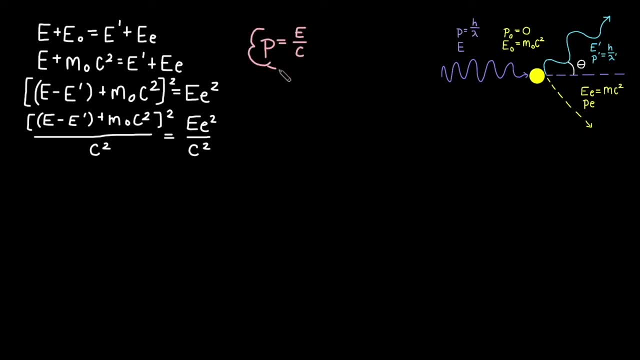 we will be able to plug in the equation: p equals e over c. In this case we have p sub e. With some algebraic manipulation we get e minus e prime divided by c squared plus two m naught times e minus e prime. 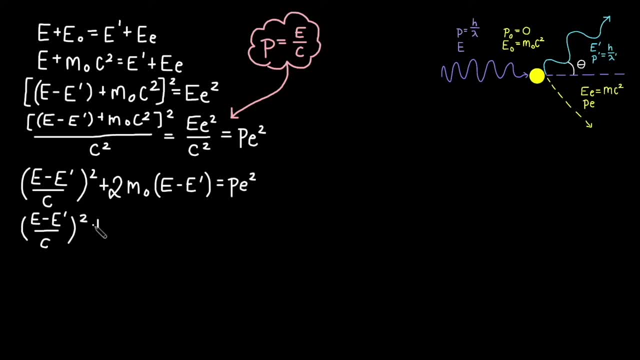 which equals p sub e squared. We can multiply the second term by c over c to get an expression that now resembles our p equals e over c equation. Now we turn to the conservation of momentum, which implies that the momentum of the photon and the electron before collision is equal to the momentum of the photon and the electron. 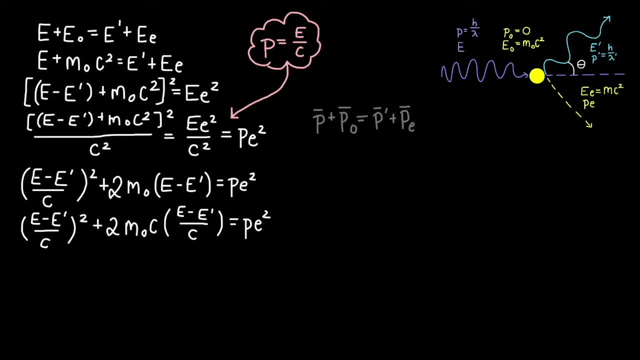 after collision. We haven't yet focused on how the momentum is a vector, meaning it has both a value and a direction. but that becomes important here. First off, we can eliminate the initial momentum of the electron, because in our scenario we assume the electron starts at rest.